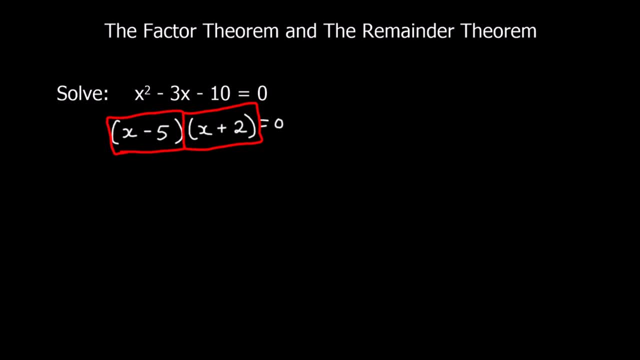 are x minus 5 and x plus 2.. If I were going to go on to solve it, I'd give my answers as a positive 5 and a negative 2.. So this is going to show us what the factor theorem is. So the factor theorem says: if x minus 5 is a factor, then f of 5 will equal 0. So 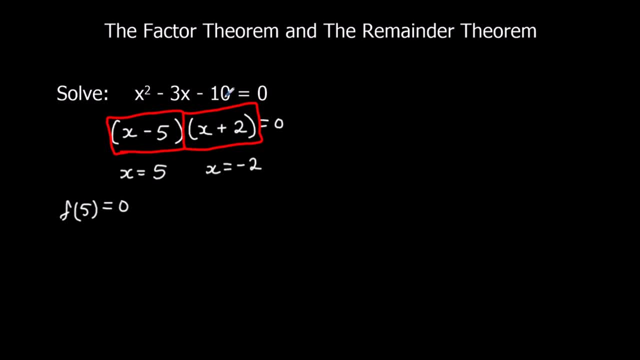 if I substitute in 5 to this, I should get a 0 out, And if x plus 2 is a factor, which it is, f of minus 2 should equal 0. So we can substitute these in and check. So if I. 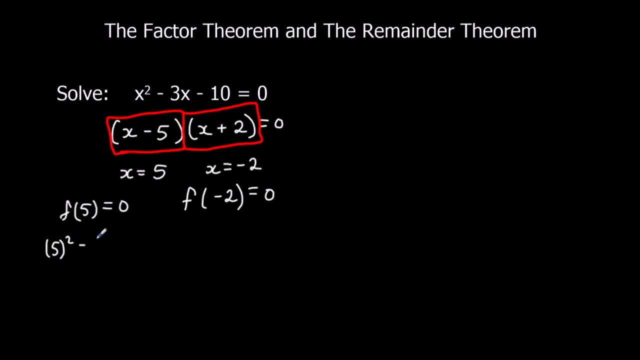 substitute in 5 here. so 5 squared minus 3, fives minus 10,, 25 minus 15 minus 10, well, that is 0.. So x minus 5 is a factor, because f of 5, if I substitute 5 in, it gives me an answer. 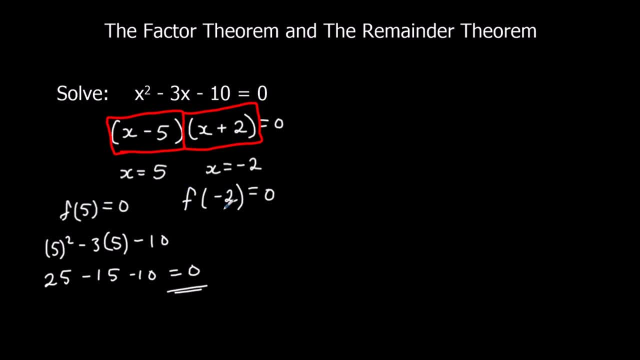 of 0.. The same thing will work if I substitute in minus 2, I'll get an answer of 0, because x plus 2 is a factor. So that's the factor theorem. So if x plus a is a factor, then 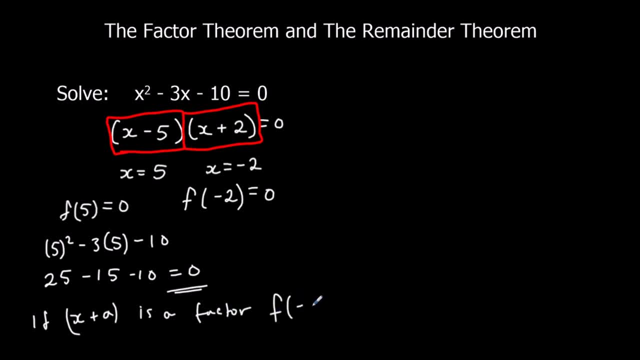 f of minus a equals 0. That's the factor theorem. The remainder theorem is slightly different. So if I did f of 2, so x minus 2 isn't a factor, so it won't give me an answer of 0.. So I'll. 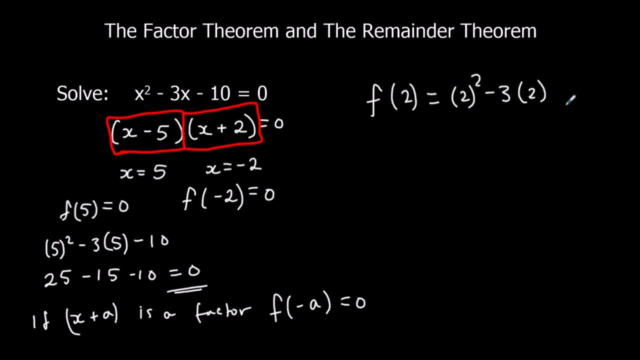 get 2 squared minus 3, twos minus 10.. So that's 4.. 4 minus 6 minus 10,, 4 minus 16, negative 12.. So what that shows us is: if I divided by x minus 2, I would get a remainder of minus 12.. So the remainder theorem says: if I divide 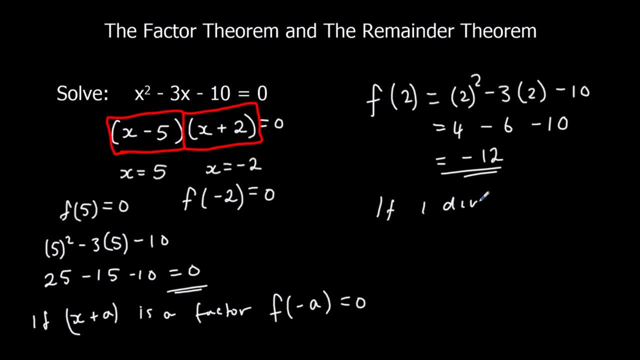 by x Plus b, f of minus b will give me the remainder. So if it doesn't give you 0 when you substitute it in, that tells you it doesn't divide by that. That isn't a factor And the answer you get is actually the remainder. 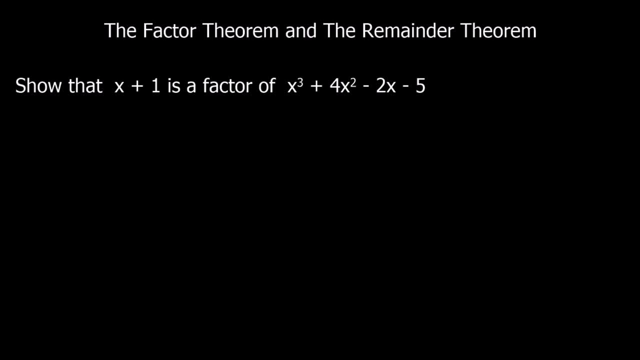 So let's look at some examples of this. So here we've got a question that says: show that x plus 1 is a factor of x cubed Plus 4x squared minus 2x minus 5.. So show that x plus 1 is a factor. So that means we: 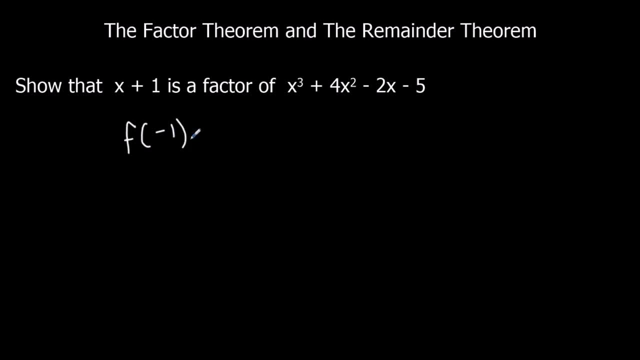 have to substitute in a negative 1.. So we substitute in the negative 1.. So we have negative 1 cubed plus 4 times negative 1 squared, minus 2 times negative, 1 minus 5.. So minus 1 cubed is a negative 1. Plus 4 times negative 1 squared, which is 4. Negative. 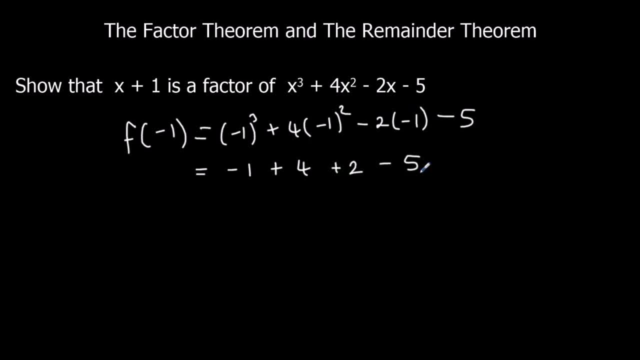 2 times negative. 1 is a positive 2. It's 5.. So we've got minus 1 plus 4, plus 2 minus 5. That equals 0.. So we've shown that x plus 1 is a factor, because f of minus 1 equals 0.. 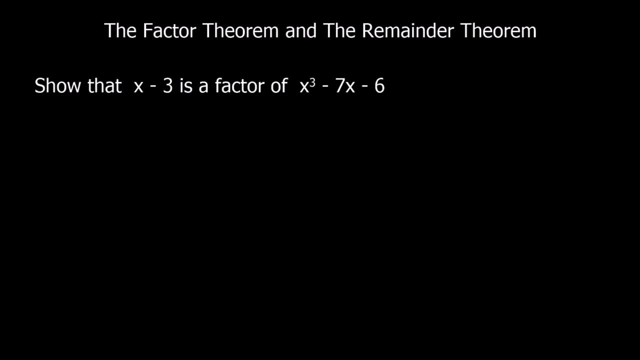 Show that x minus 1 is a factor. So we've shown that x plus 1 is a factor, because f of minus 1 equals 0.. Show that x minus 3 is a factor of x cubed minus 7x minus 6.. So if x minus 3 is a factor, 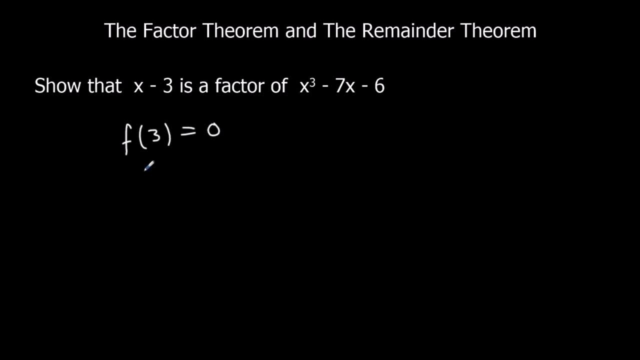 f of 3 must equal 0. So 3 cubed minus 7, 3s minus 6.. 3 cubed is 27.. 7, 3s are 21.. And again that equals 0. So 27 minus 21 minus 6.. 27 minus 21 is 6.. Take away another: 6 is 0.. So x minus 3 is. 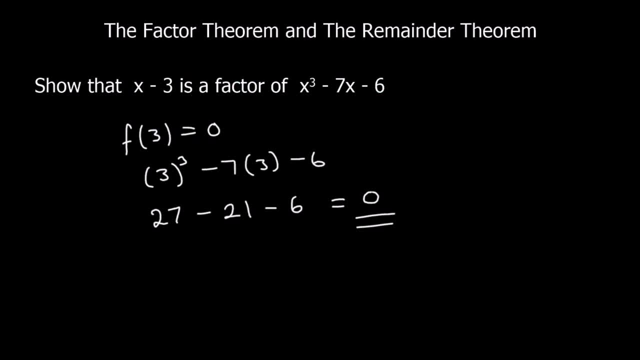 a factor, because f of 3 is 0.. Okay, find the remainder. So this time x minus 2 isn't going to be a factor. Find the remainder when x cubed plus 4x squared minus 2x minus 5, is divided by x cubed minus 5.. So we've. 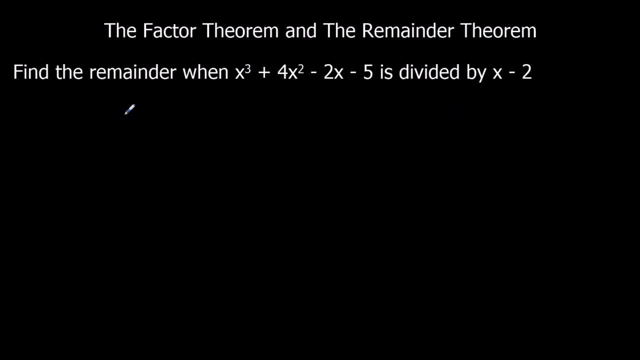 got x minus 2.. So we're going to do the same thing. We're going to substitute in 2.. And this time it's not going to give us an answer of 0. We just need to know what the answer is. So we substitute in the 2.. 2 cubed is 8.. 4- 4s are 16.. Minus 4 minus 5.. So that's. 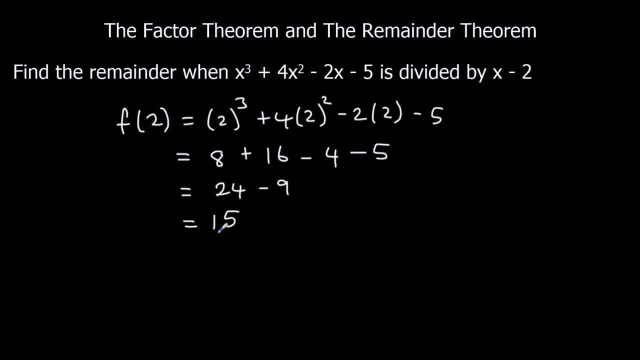 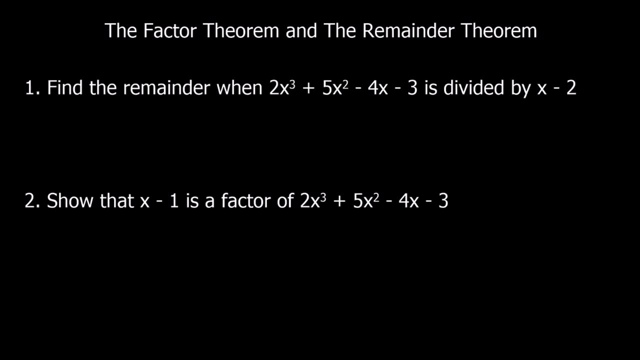 24. Take away 9, which is 15.. So the remainder, when x cubed plus 4x squared minus 2x minus 5, is divided by x minus 2. It's 15.. Okay, here's a couple of questions for you to try. So pause the video. give them a go. 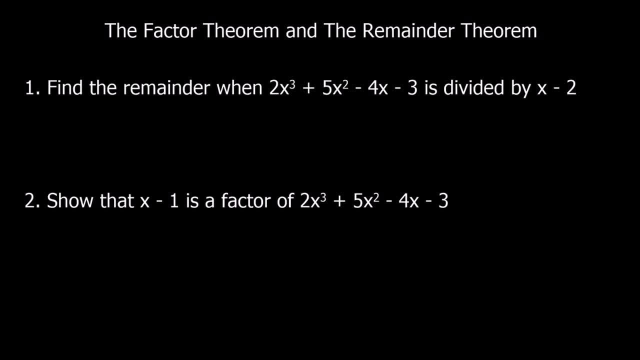 and then I'll go through the answers after. Okay, so firstly, we're going to find the remainder when we divide This function by x minus 2.. So we're going to substitute in 2. And we'll see what we get out. So 2, 2s cubed plus 5 times 2 squared minus 4, 2s minus 3.. So 2, 8s are 16.. 5, 4s are 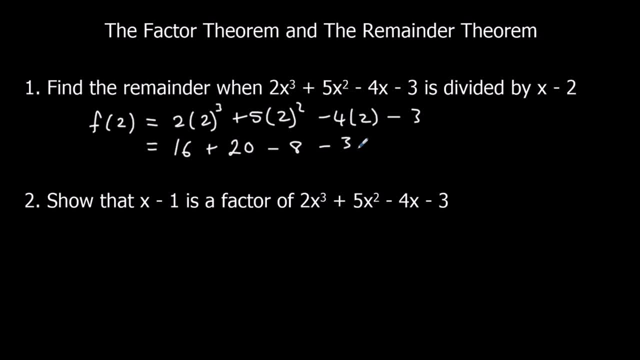 20. Minus 8 minus 3.. So that's 15.. 36 minus 11,, which is 25.. So the remainder is 25.. Secondly, show that x minus 1 is a factor. So that means we need to substitute in the positive 1. And it should equal 0..